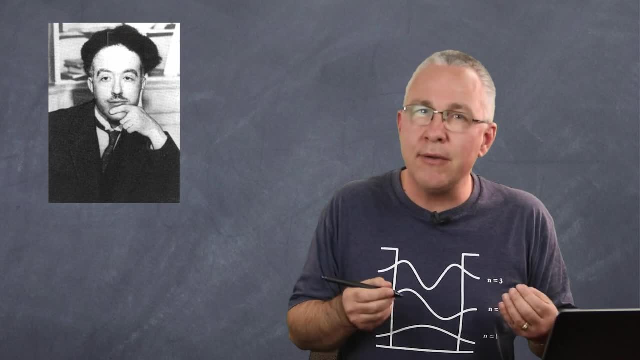 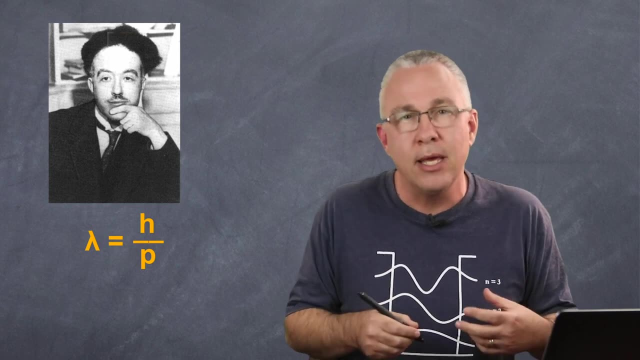 the electrons existed as waves and he derived what we now know as the de Broglie relationship, That is, the wavelength is equal to Planck's constant divided by the momentum. Now that means, interestingly enough, of course, that photons of light can have momentum. but critically is that? 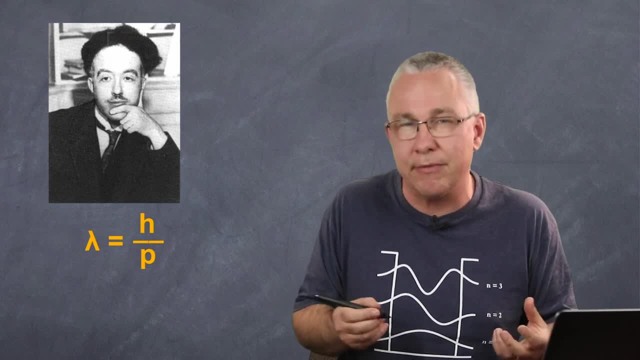 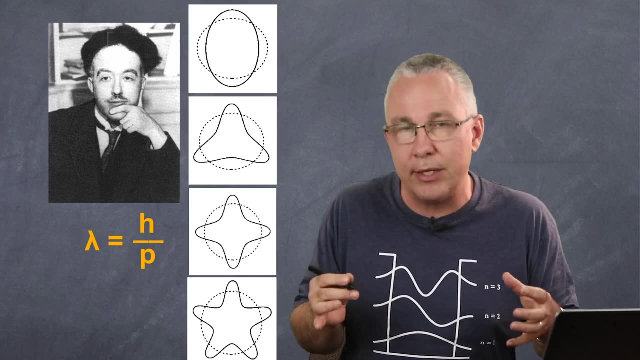 now, electrons that have momentum, as we classify them as electrons, are not as important as the electrons that we classically think of them, but now have an associated wavelength, And he came up with the idea that they exist in discrete energy levels because they were like standing waves around. 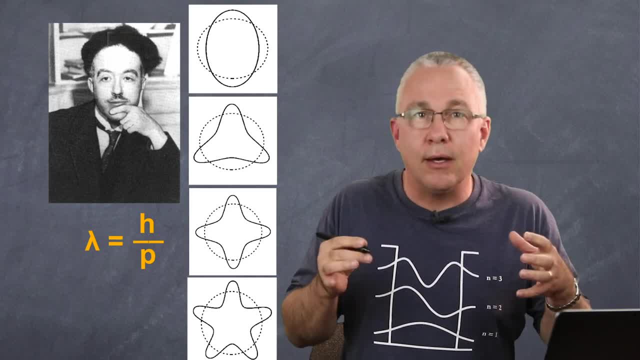 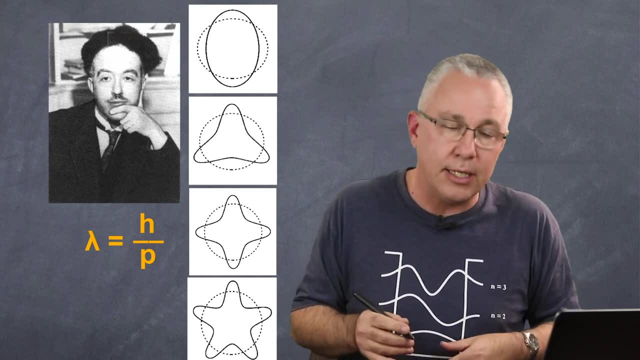 the orbit, And if you have standing waves, you can have discrete waves. as a result, You can have harmonics at higher energy levels, because they're in different resonances, And so what we have here is our understanding of de Broglie. But then is where Schrodinger, where it comes in, And he 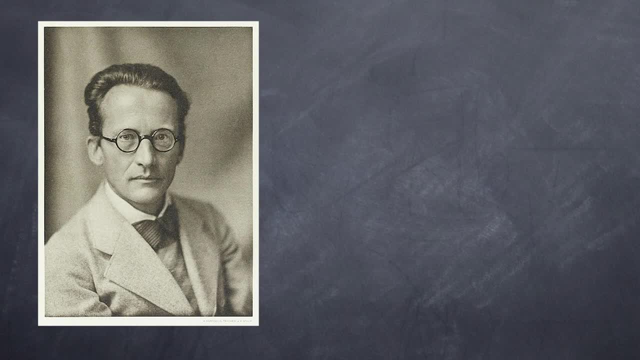 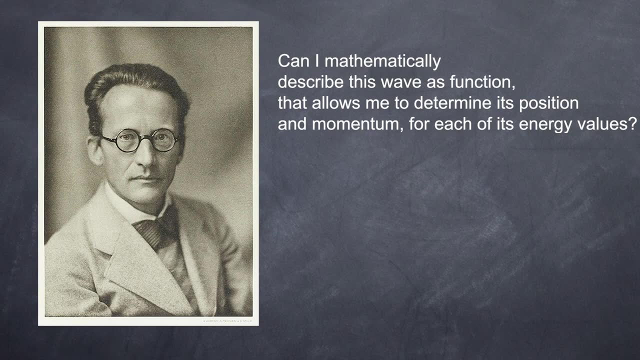 really asks two questions. The first is: if it is a wave, then can we use mathematical functions to describe these waves that exist in terms of the electrons around them, And therefore from this can we extract information such as their momentum and their energy values? Secondly, can this function then explain all the orbits that 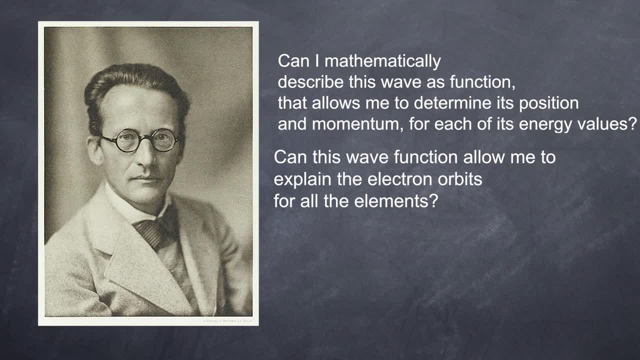 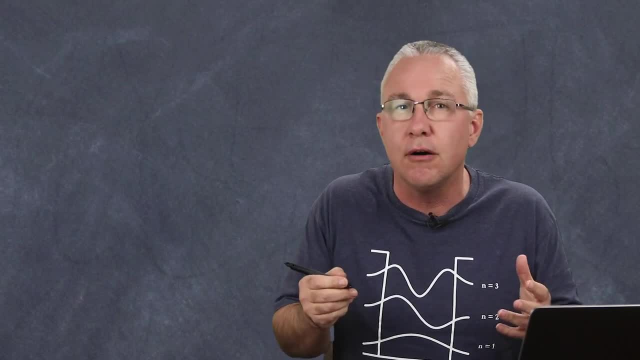 the electrons exist not only for hydrogen, but also for other atoms as well. Now, the beauty of equations is that they allow you to determine various features of what you're particularly studying. So, in terms of particles, you're familiar with equations such as f equals ma. 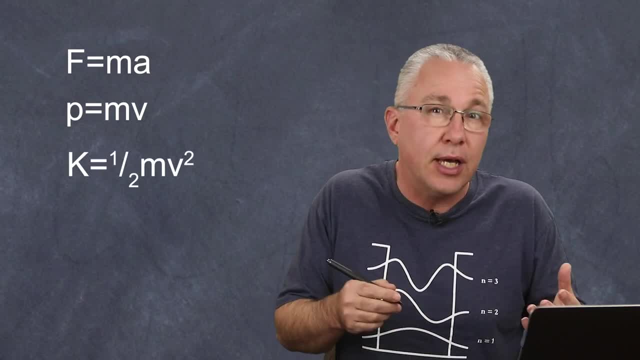 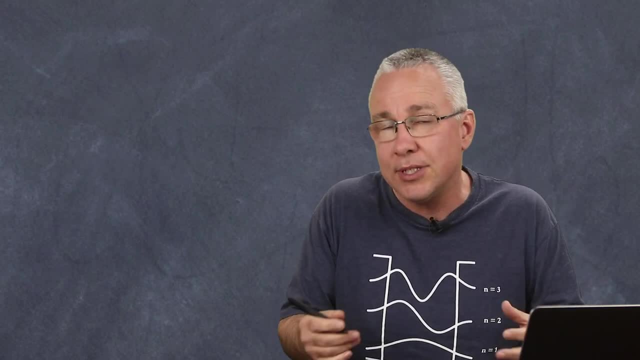 the momentum equals mass times. velocity energy is equal to half mp squared in terms of kinetic energy, and so forth. In other words, equations allow you to make predictions of how a particle behaves, And the same is true also for waves. So what Schrodinger did? 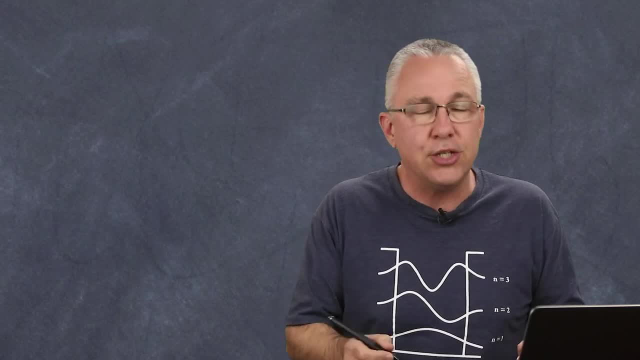 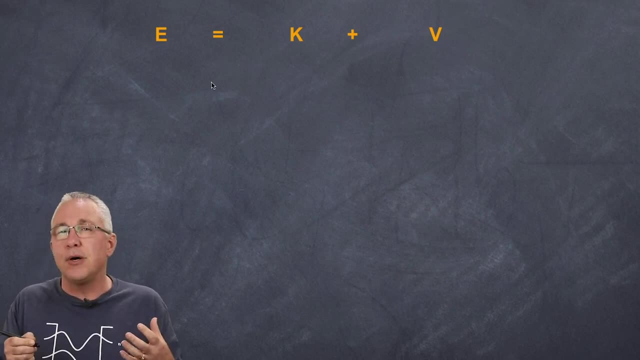 he started off with the concept of the conservation of energy. Now you all know that the conservation of energy basically says that the sum of all energy is a combination of both its kinetic energy and the residence of the energy mass. And in addition to that you can also have the 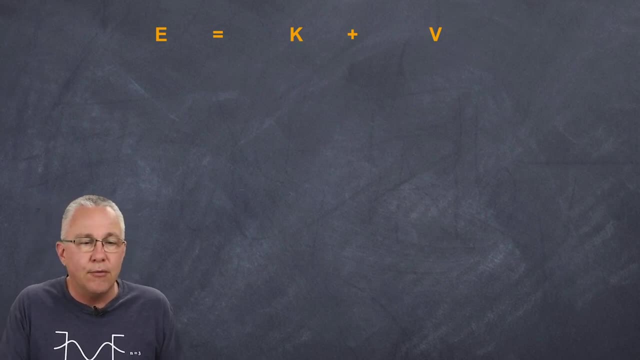 energy and the potential energy. And if we were to write that as a mathematical formula, we have a half mv squared plus v. Now here the v is another way of describing the potential energy. So when we look at a quantum state, this electron, 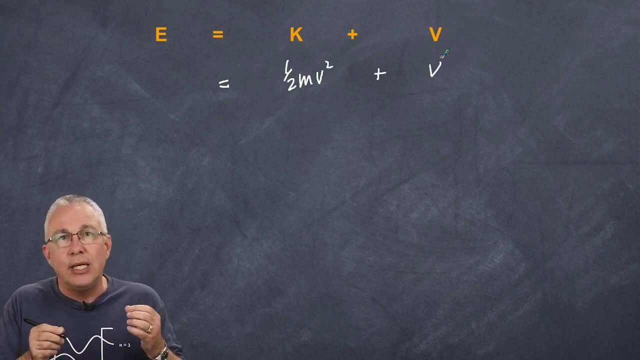 that is a particle and wave duality. we can determine its total energy by looking at its kinetic energy and also its potential energy. Now, half mv squared is something that you're familiar with, but in this case this looks as a particle. How can we somehow incorporate the concept of the fact that we're 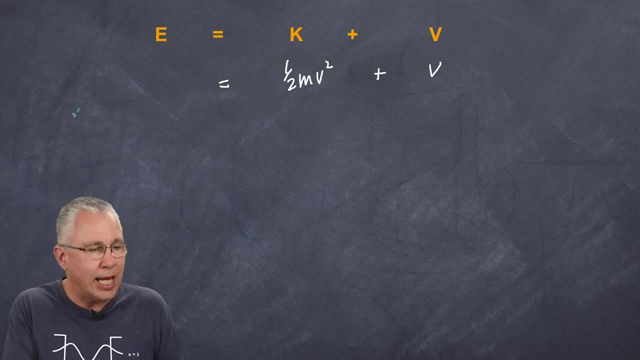 dealing with a wave, And this is, of course, where we get de Broglie's relationship. De Broglie's relationship simply says that the wavelength of a wave is equal to the Planck's constant divided by the momentum p, But we don't. 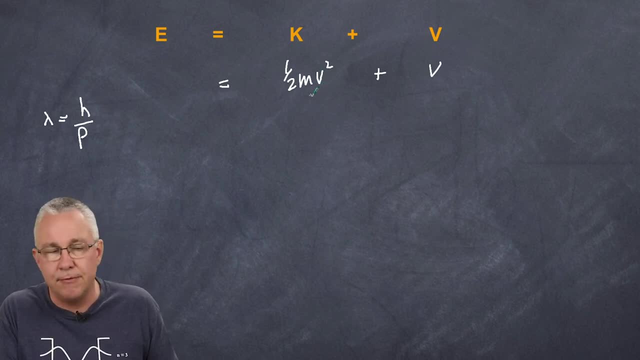 have a momentum here, But you know the momentum is mv, and so another way of writing half mv squared is to write half mv squared plus half mv squared. It's simply saying what we have is, in this case, p squared over 2m. That's the 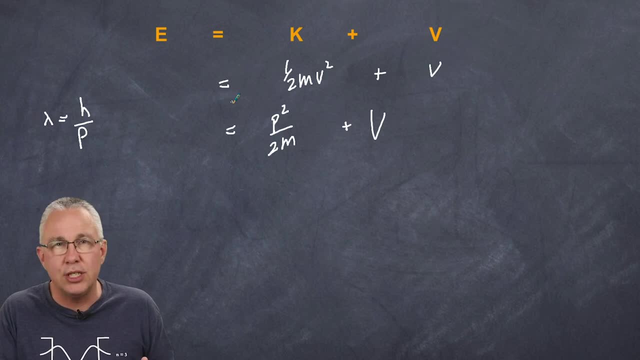 same thing. And now you can see what I have is that the energy is now described in the terms of momentum and its mass. And remember, de Broglie's relationship says the momentum and the wavelength are intricately connected. And so now you can. 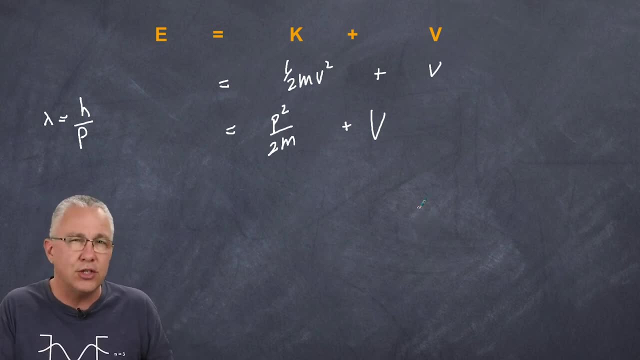 see, we can embed the concept of a wave in this conservation of energy, And that's what Schrodinger did. But he also introduces the concept of what we call a psi, Which is basically called the wave function. Now, what is that, And I'll mention. 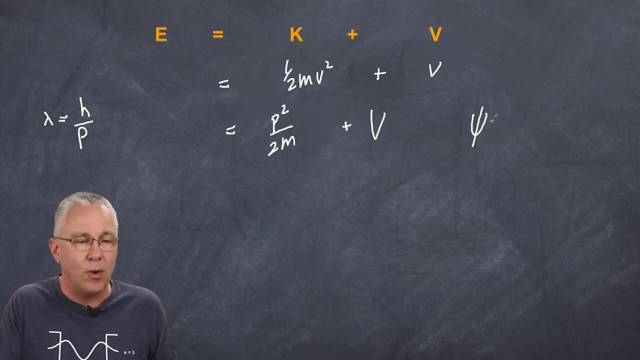 this right now. Psi is simply a sine wave. Now, one way I can write this wave is in terms of a sine function, And I call it sine, or a times sine, outside of kx minus omega t. Now how is that? Well, we know what a sine wave is. This omega t tells us in: 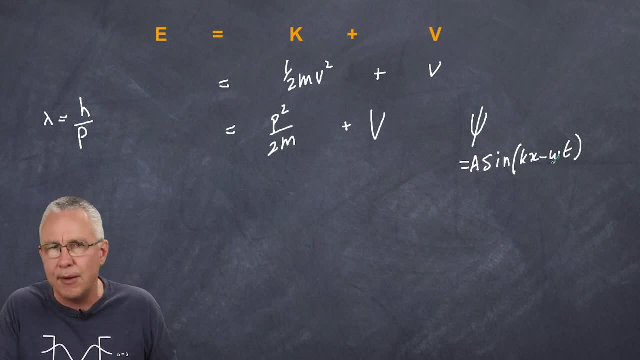 terms of how its velocity is happening with respect to time. It's a sine wave that's moving. k changes the wavelength and therefore the frequency as well, A changes the amplitude, And so now what we have here is a function that describes a wave, And in 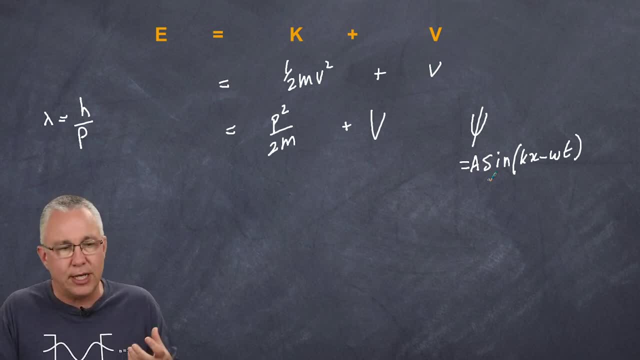 this case it's called psi, And we call this the wave function. Now, strictly speaking, the wave function is a little bit more complex than that, but in essence it describes a wave, And the beauty about this, of course, is that it also allows us to make predictions. It tells us everything about that wave. 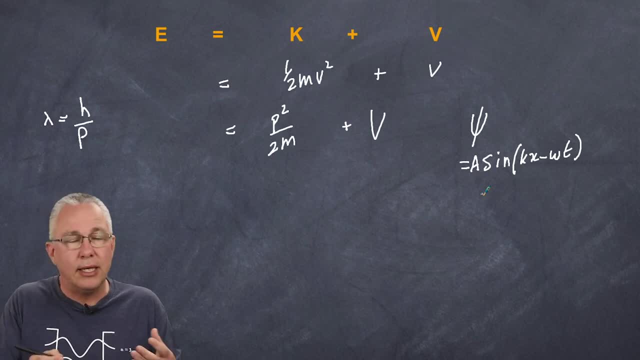 including the momentum. Why? Because the momentum is basically related to the wavelength, but what we don't know necessarily is a position and, as you know, a wave doesn't have a discrete position, it is actually a wave. Now, when he puts this all together, he gets this particular function and you get E. 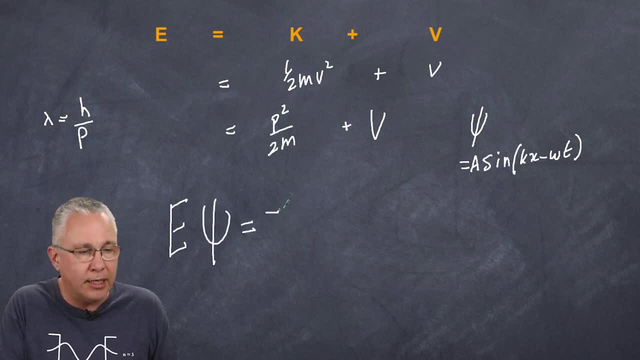 multiplied by psi is equal to negative h bar over 2m multiplied by the second derivative of psi with respect to the displacement x plus the potential energy multiplied by psi. Now this is what we've referred to as the time-independent Schrodinger equation. Now it looks complex, but let me just really break it. 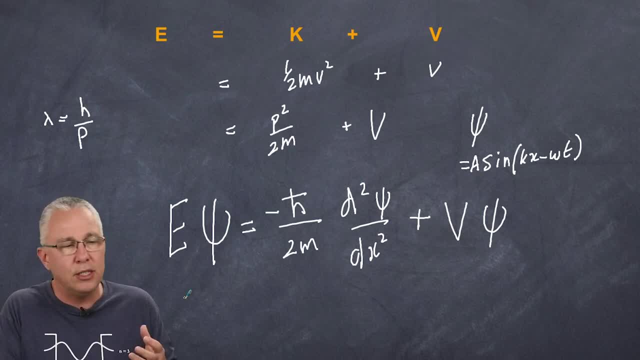 down for you What he's really saying, look, is, if I want to know the energy that the electron is allowed to have in terms of the psi here- that's what I want to work out, that's what I want to determine about my electron- then I 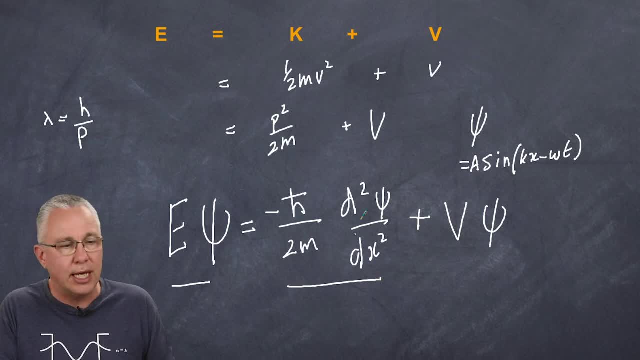 really want to know the energy that the electron is allowed to have in terms of the psi here. that's what I want to determine about my electron- then I really have just two aspects that I need to use, and that is the kinetic energy, which is: 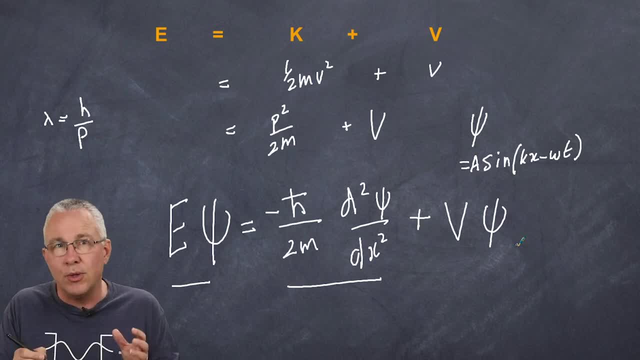 the first half of the equation and the potential energy. So, in other words, if I can find solutions to psi, I can determine the features, such as the energy, of my system, and that's the critical thing about Schrodinger's equation. Now, 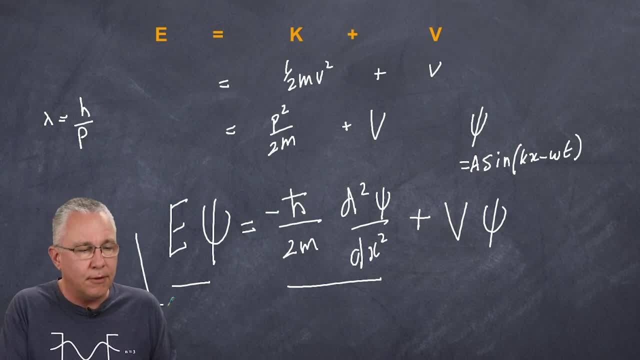 the beauty about this equation, too, is that this form of that we have right. there is actually a wave equation in itself. In other words, it's a wave actually describes, at least in the mathematical sense, a wave. Now, what does? 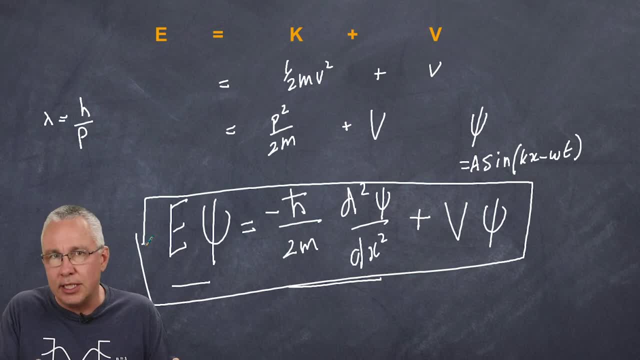 a wave look like. Well, Schrodinger didn't know, others didn't know, but at least in a mathematical sense this is a wave. The other thing I want to touch on too is that this psi- if I took at all the possibilities of psi that we can have, and 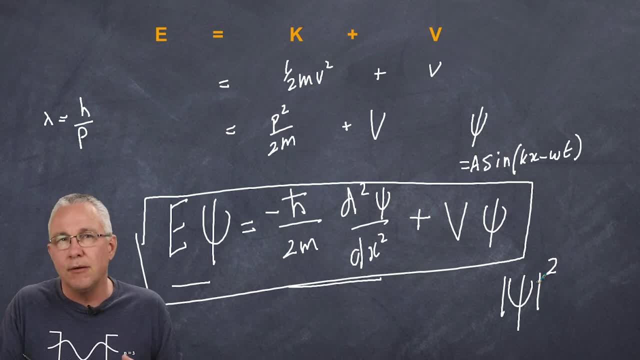 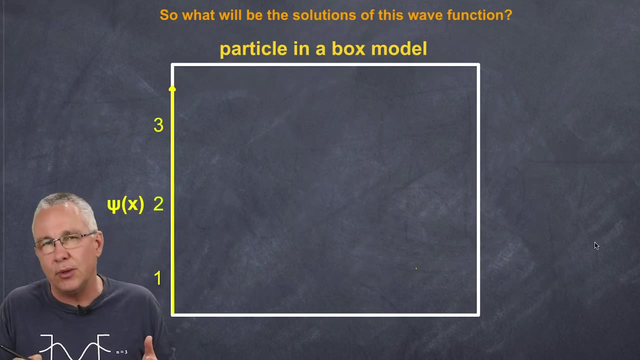 then we square that in terms of all the possible versions of psi, then what we end up is getting the probability of where the energy of the electron is allowed to exist or where the electron actually exists, and we'll refer to that in a moment. So what we now come to is the idea of a particle-in-the-box model. Now, 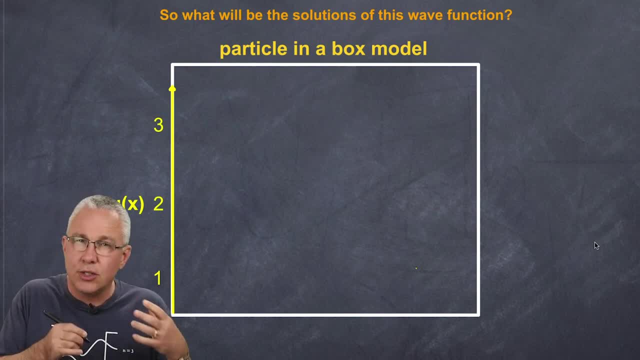 of course, our wave, that is, our psi function that is described within the wave equation, isn't allowed to roam anywhere. It's in the confines of the atom, And so what we want to do now is look at that. what happens when we place? 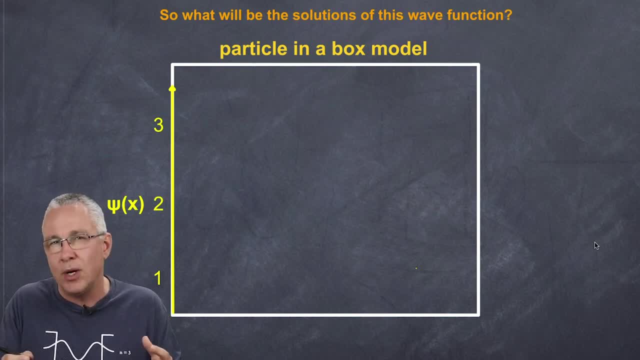 a confinement in place. How can we make this in terms of a standing wave? How can we show that that's a standing wave? How can we show that that's a standing wave? And so what we have here is an analogy which is referred to as the particle-in-the-box. 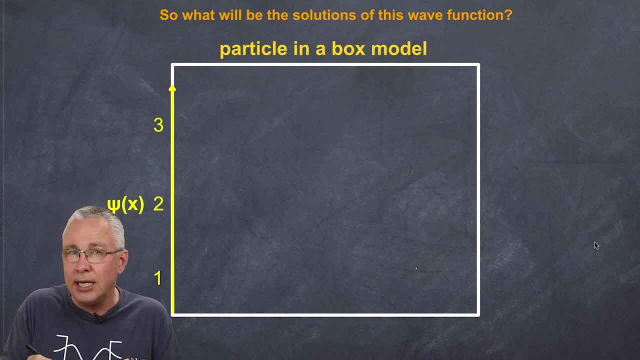 And what we do is now we look at it just in one dimension. In reality, Schrodinger's equation describes the electron-wave duality in three-dimensional space, But what we want to do is just look at this in a simplistic sense, in a one-dimensional. 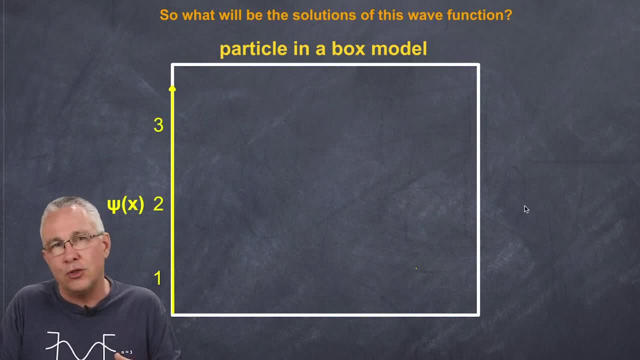 space And if we actually try to work out the solutions to give us the energy, we end up getting a formula that looks like this. Now, what again this formula looks like is quite complex, but let me just break it down for you. If you look at all, 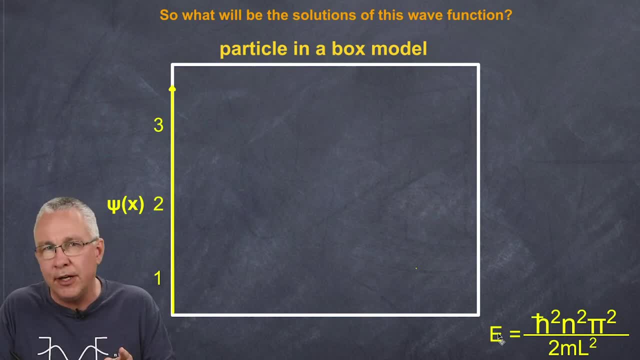 the variables that are in that equation. there is only one variable there that can actually change, And that is N, which is the energy levels, that is, the discrete energy levels: h, bar, which is the first one, pi 2,, obviously, m, which is the mass, and L, which is the. 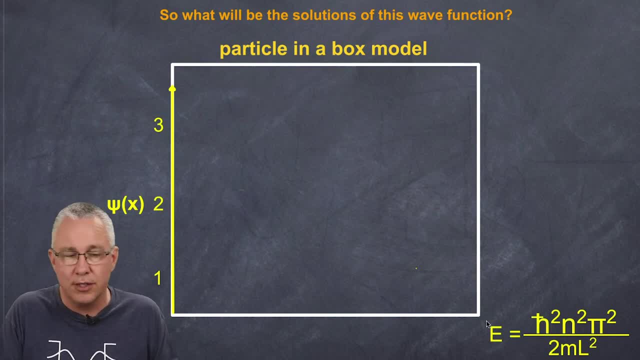 length of the box here that we have across here are all constant. So what is this saying? says that the energy of this wave that Schrodinger's equation describes when confined in a box is a standing wave of discrete energy levels. And so what I? 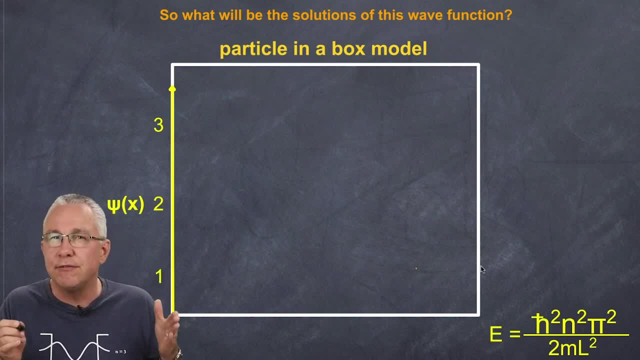 want to do now is show you what happens to our waves when we confine them in the box. Now, the electron cannot exist outside the box, and so will we say it has no energy value outside the box. But inside the box we can have it existing. 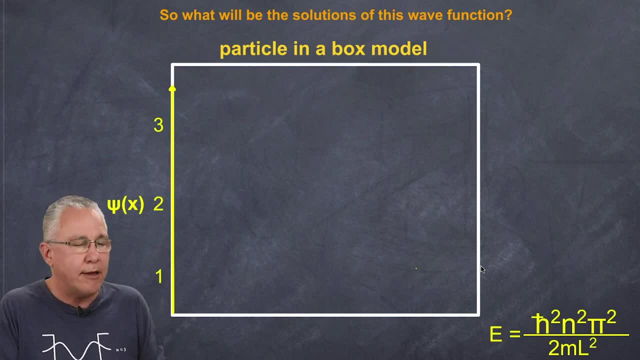 but remember, it exists in terms of a wave, a standing wave. So when we do n equals 1, we get the classic fundamental wave. That's the e-value. It has discrete energy value. But if I try to increase the energy, the only way I can increase- 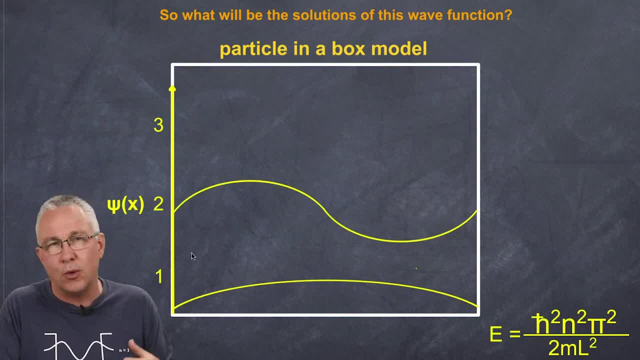 the energy is when n equals 2 and, as a result, we get a second standing wave, We get the next harmonic and you can see we have a node right in the center. Then, of course, if I increase that to 3, I'm going to have two nodes in the middle. If we 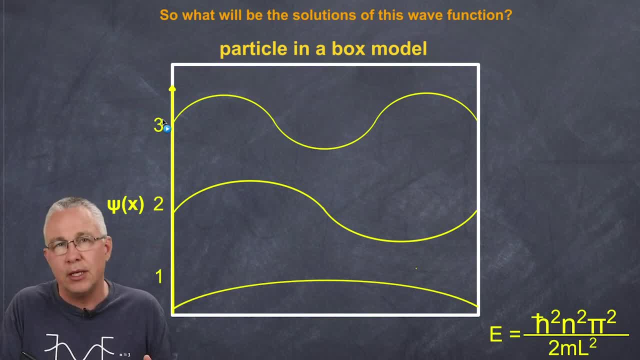 look at this wave, this psi function, and we look at all the possible psi functions and we square it, we get what we refer to as the probability of that, And that is Max Born's contribution. He looked at this and said: look, the wave that is Schrodinger's equation is describing is not a wave in terms of just. 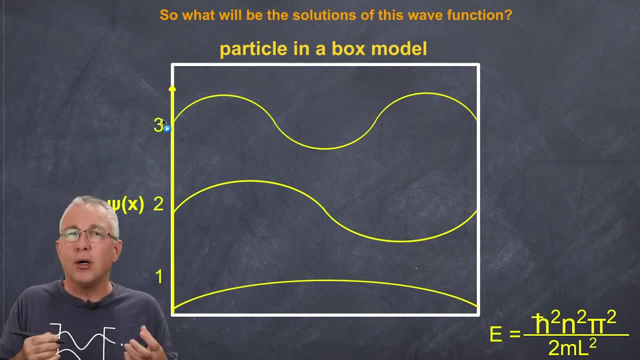 in physicality, a wave, but a wave of probability. Now let me explain what that means. So the first thing we're going to do is we're going to look at the right hand side, I'm going to place this axis and I'm going to see: here, this is the psi x function and it's squared, And I'm just 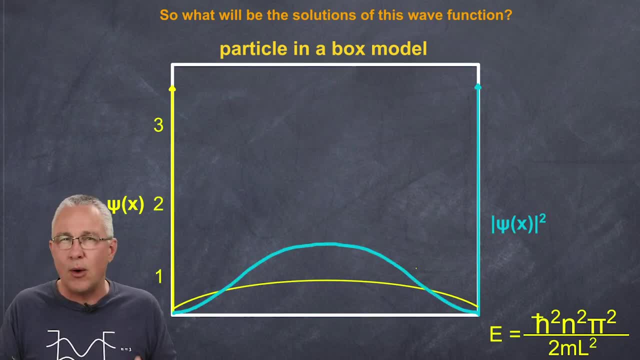 going to look at one. If we square that particular function, we get this. Now what does that mean? It means that if I were to open up the box and look inside the box while this electron is existing as a wave, the likelihood of me finding the 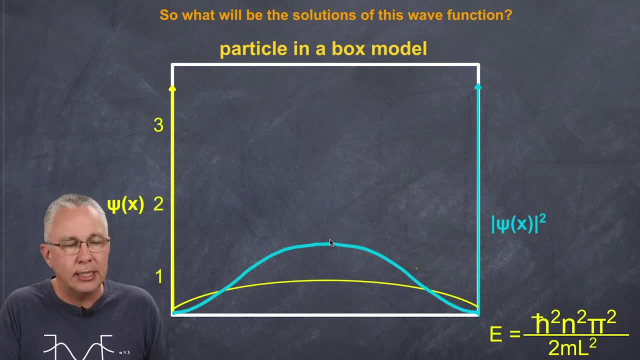 electron in a particular place would more likely exist in the middle and less likely at the edge. Now make sure you've got that in mind At the very edge. it's very unlikely for me to find the electron at the very edge, and certainly not outside the box. This is where the node is, But it's more. 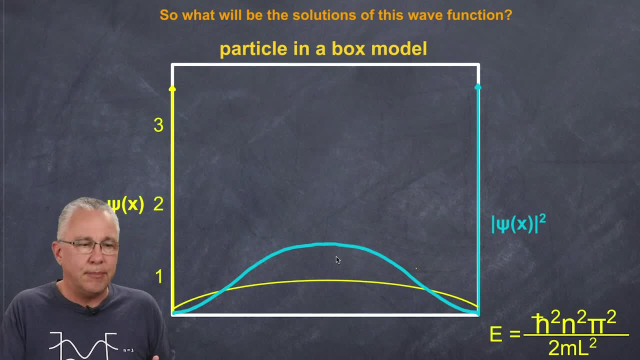 likely to be in the middle. If I close the box and open up again again, it'll be more likely in the middle. This is a probability graph. In other words, it's the greatest probability is in the middle. But now let's have a look at. 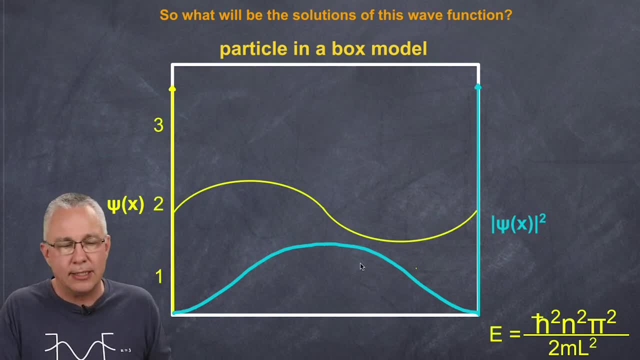 energy level 2.. If I square that, I'm going to get not that but that. Now this is where it gets really interesting. That means if I open up the box, the likelihood of me finding the electron in, let's say, this box is greatest at these points here where the amplitude of this curve is greatest. but 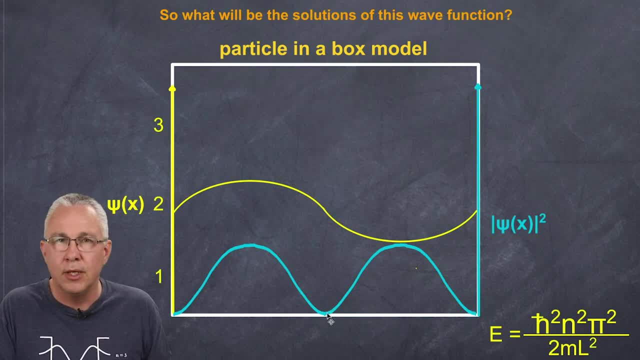 nothing at the edges and nothing in the middle. In other words, if there's an electron existing in that box, I will never find it in the middle if I were to open it up and look at it. Now, that's a bit weird, Because electron seems to want to be able to be existing in any one place If 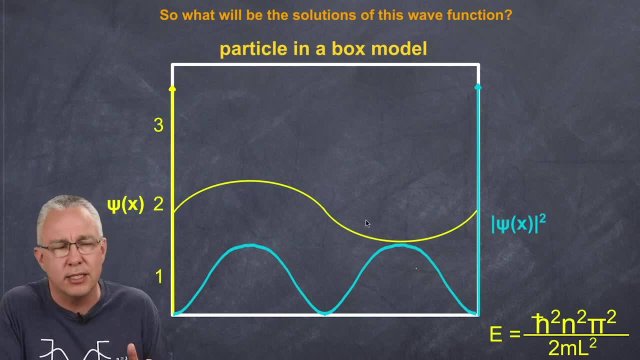 it wasn't literally just a particle moving around the box, surely I would find it somewhere, sometimes in the middle. But remember, this exists as a wave when we don't observe it. It only exists as a particle. when we observe it, We say that the wave function collapses. What about when we increase the energy? 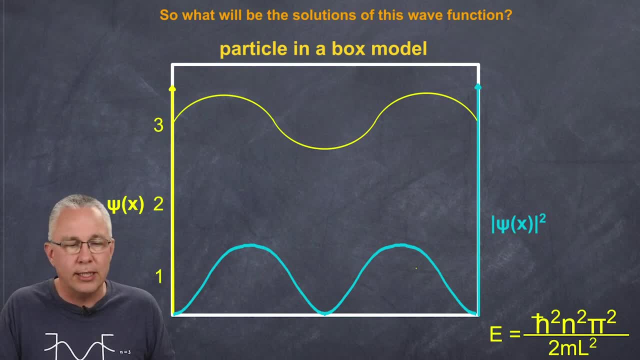 level not from 2 but to 3? Well, it's not going to look like this. it's going to look like this. now, what we get is we have these three antinodes of basically the peak, the likelihood, the probability of finding the electron there when we observe it. 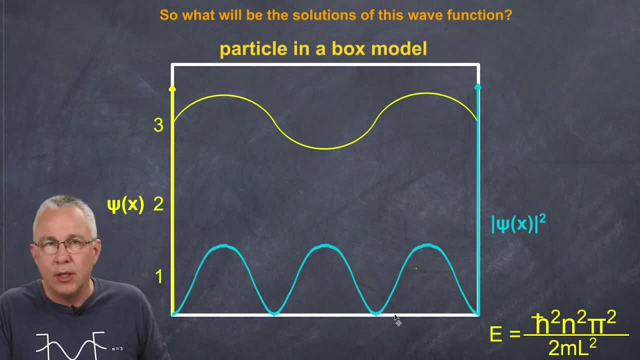 and no probability in between, which is, again, not intuitive. We would expect the electron to be able to exist in any place, but that's because we have this idea. the electron is a particle and we just can't observe it. No, no, if you don't. 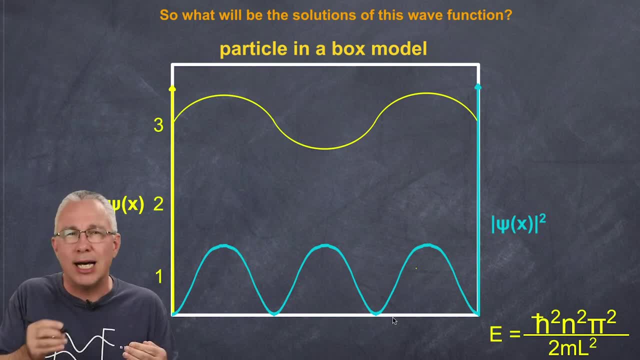 look at it, it's existing as a wave. Remember this wave-particle duality is what it's doing naturally. So, in other words, it's acting as a wave. so it's acting as that yellow wave, but the probability of finding it when we 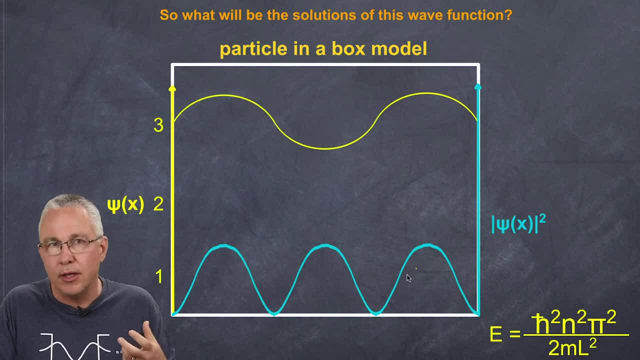 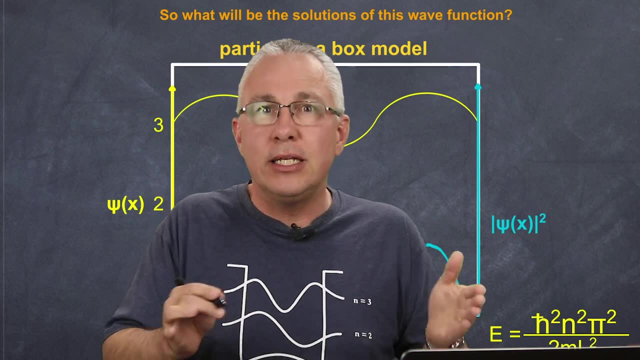 observe it when it becomes a particle, is based on the blue graph. Now, of course, this is only a one-dimensional model. In reality, it's a three-dimensional model, And so what does that look like? Well, that leads us to an understanding of the 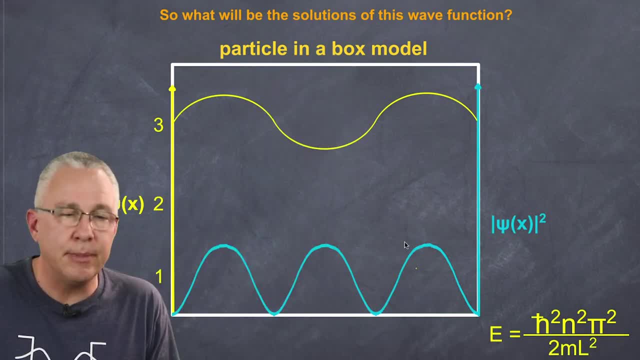 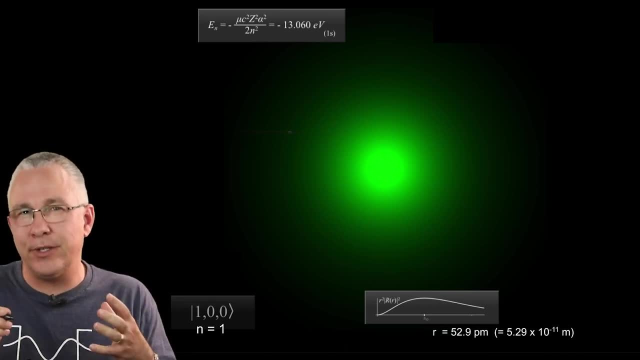 concept of a particle of electron clouds. If we look at a three-dimensional, we get something called an electron cloud. Now it's important to note the electron cloud is not a physical reality in the sense that if you were to have some sort of super, 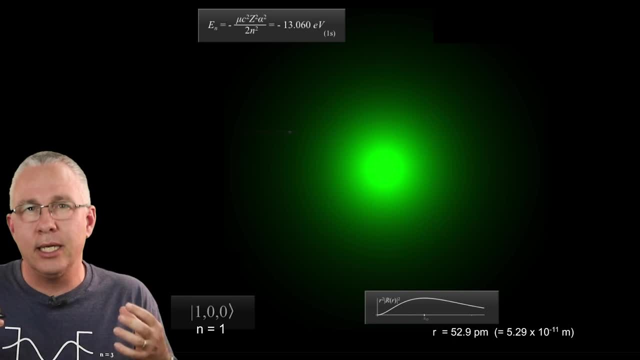 super microscope and looking at that and we don't have that ability. it's not. you're going to see a cloud. in that sense, This cloud is actually a probability function that allows us to say where is likely we're going to find the electron. So the thicker the clouds are. 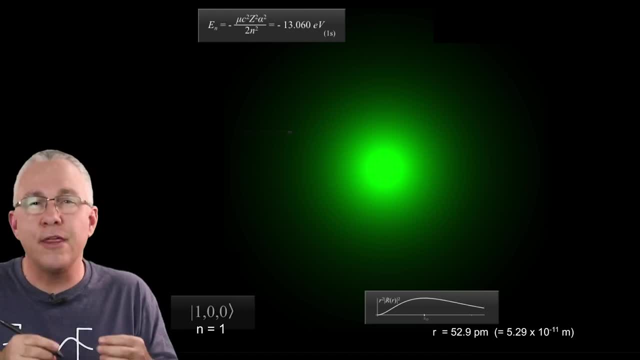 under-speak. the higher the probability of finding the electron there. The thinner the cloud, the less likely to find the probability. Now, if we took this one cloud here, this is the lowest energy level, where n equals one. this is what the 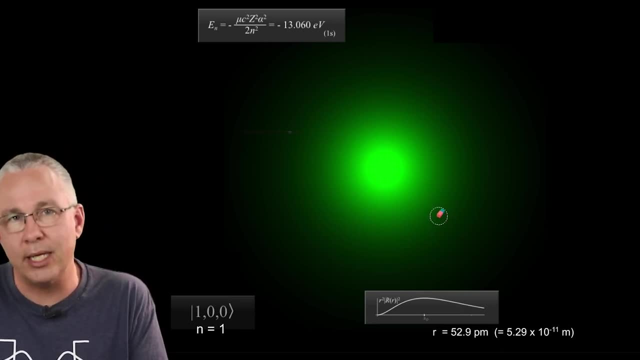 number here is: we have our energy level up here, which is how we can calculate using Schrodinger's equation. If we look at cross-section of that, you get a graph that looks like this, In other words, this particular radius right here. 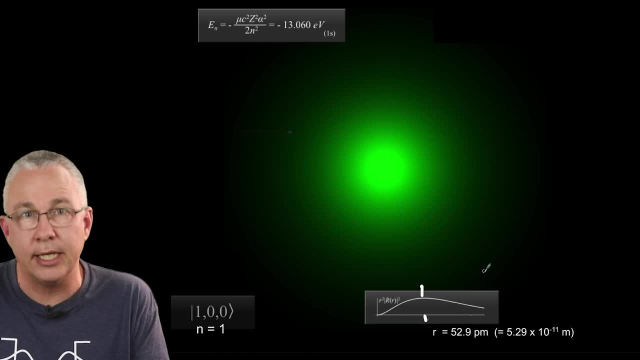 gives us the highest probability of finding the electron here. Now, the fact is that the cloud looks like it's thickest in the middle, but it's actually a little bit thinner at the edges, because you're not going to find the electron right at the nucleus Because of the way that the sphere works. 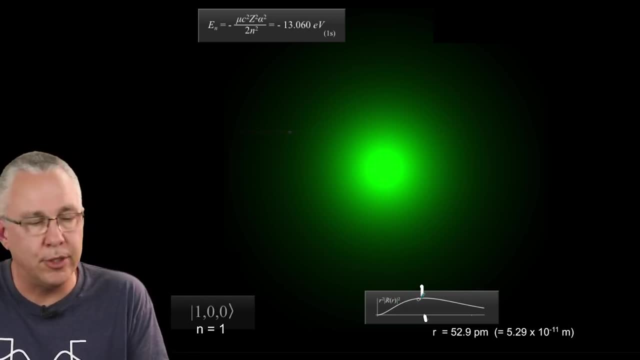 you're going to find that it's a certain distance away from the nucleus that you can find the greatest probability, But then of course it goes lower. Now, interesting to note here is that the probability that is greatest is at a radius of 52.9 picometers. That happens to be Bohr's radius for the first. 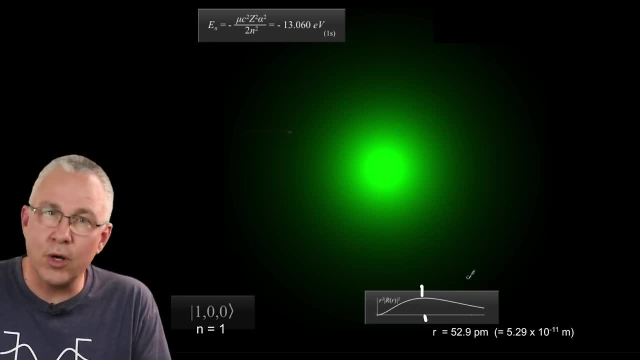 energy level for hydrogen. But what Schrodinger's equation does is says: look, that's the likelihood of finding the electron there, but you can find a possibility of the electrons being further away or closer. It's just more likely to find it at that particular radius. What about the second energy? 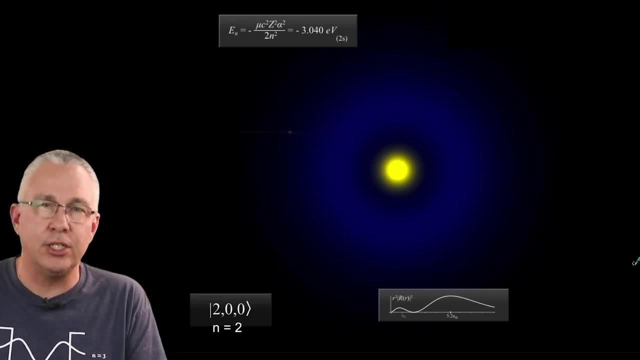 level. Well, here now, like our particle in the box at the second energy level, where we had a space in the middle where you were not going to find the electron. In this case, you can see, I have two spheres and we have a section in the middle where we are not going to find the electron. 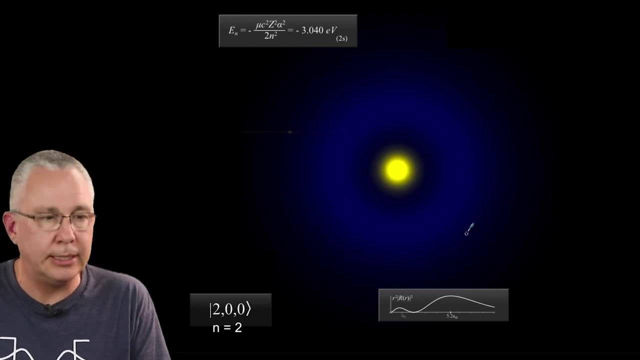 Again, this is all based on probability. So density here represents not a physicality but the probability of finding the electron where we would try to observe it. Important thing is is that this is a mathematical function. The electron is a wave. It's not buzzing around fast and fast and producing this. 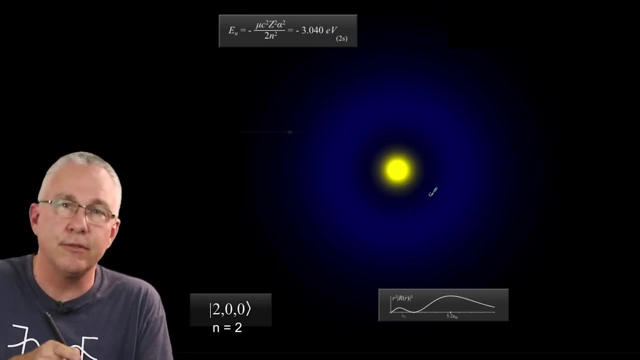 cloud. Now, if you were to observe the electron, you're going to find the electron there as a particle. but if you were to not observe directly the electron, then you're going to see it as a wave. Now Schrodinger's equation along: 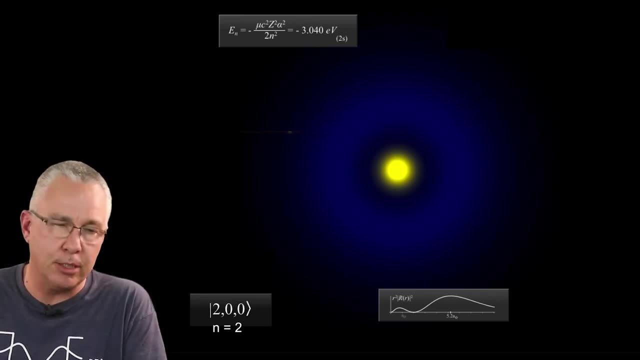 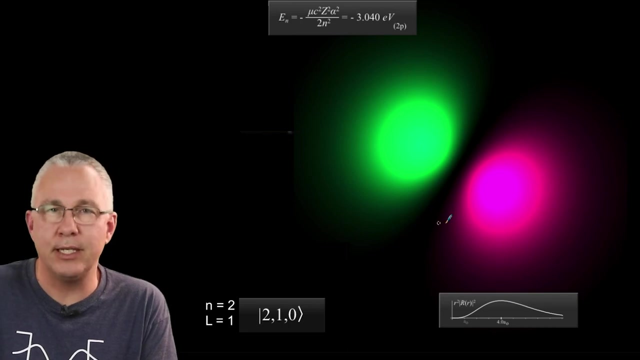 with Pauli's description of what we call the exclusion principle, is that we allow the existence of other possible orbitals that also have the energy level of negative three electron volts, And so we have this particular cloud configuration here, And in this case we have these sort of two dumbbells. Now, in this case, I've 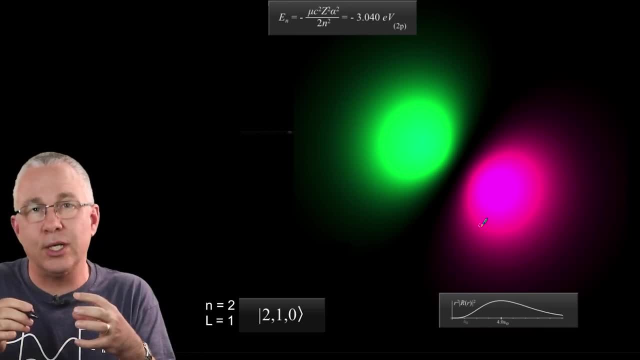 only represented it in one axis, but in the actual fact we're going to have two other axes. So in this case we have these sort of two dumbbells. Now, in this case I've only represented it in one axis, but in the actual fact we're going to have two other. 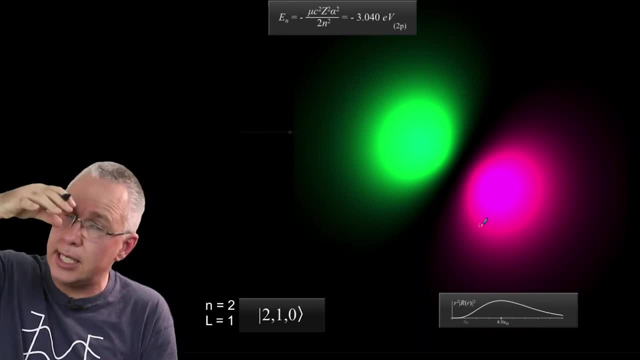 two sets here, One in the X, one in the Y and one in the Z, so to speak. And so again, these are all negative three volts And what we now get is orbitals. But the important thing here again is is that these clouds represents probability. Now, 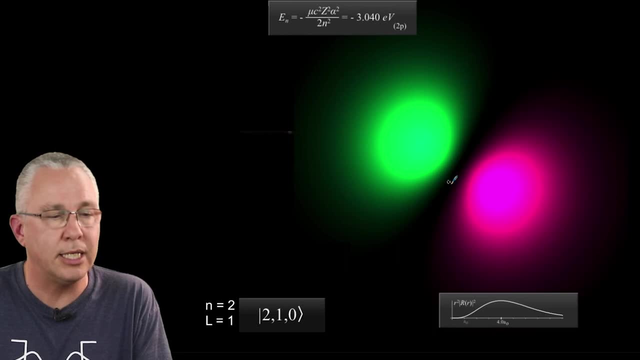 what's interesting to note, though, is that the fact that in the space here we have nothing. So if an electron can be described in this particular orbital and the electron can be described in this particular orbital as the probability- and remember, this can apply to a single electron. 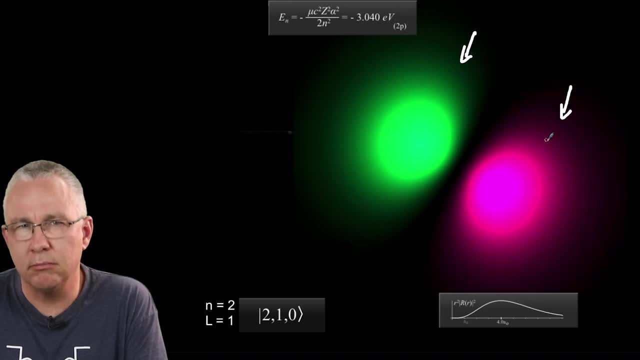 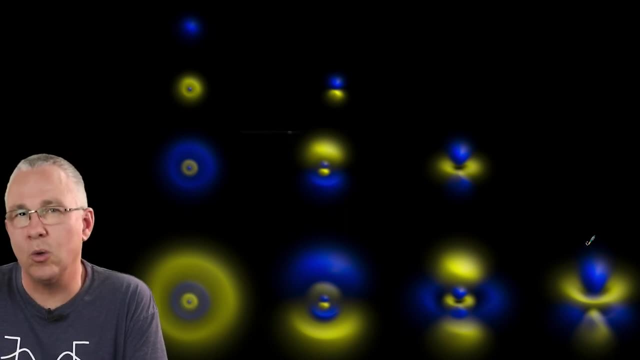 then how does it get from there to there With the gap over here? Now, if we go further, you can see here a quick setup of the different possible orbitals. These are all in one plane at this stage. So, for example, we have energy level one. 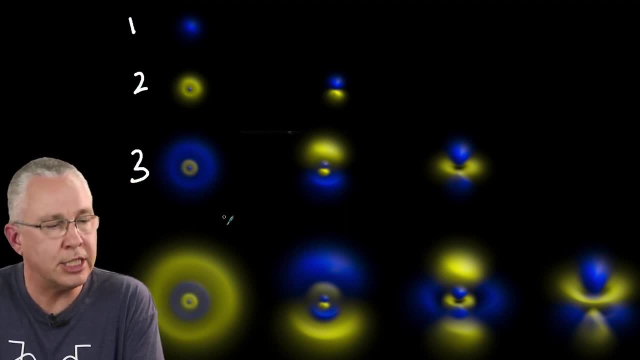 over here we have energy level two and three. You can see the spheres that are going out. And then of course I have the two dumbbells, so to speak, for the P orbitals, which are in this case only in that direction, But of course they can be. 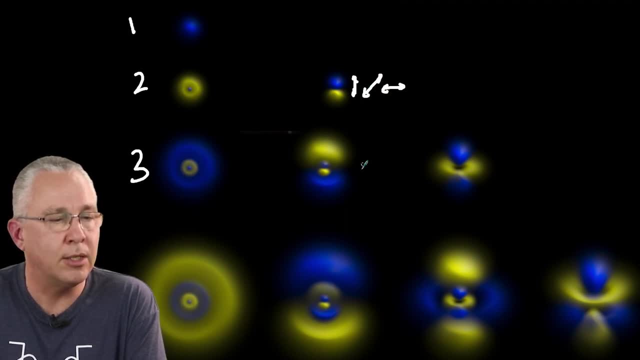 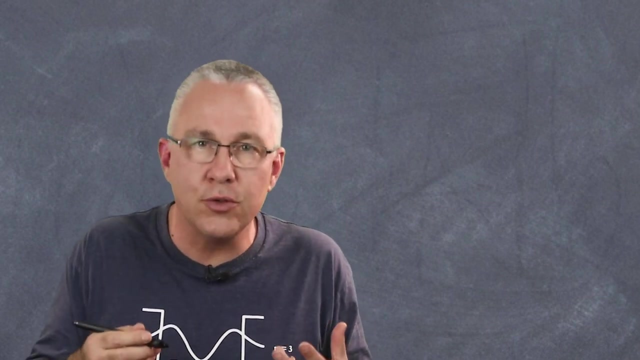 also be in that direction, and in that direction as well. And then we also have the D and so forth, And again you can see they have these specific shapes associated with them. Remember, they are probability functions. So what can we really conclude here? What is the significance of Schrodinger's equation? 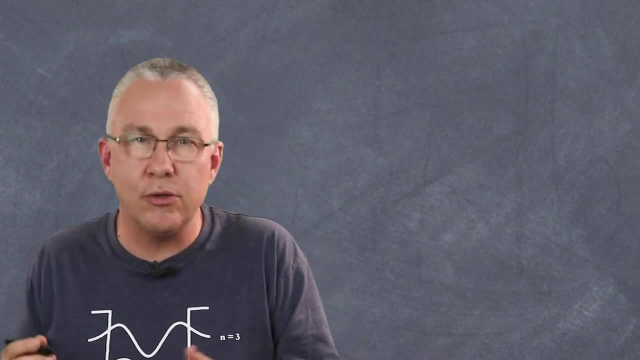 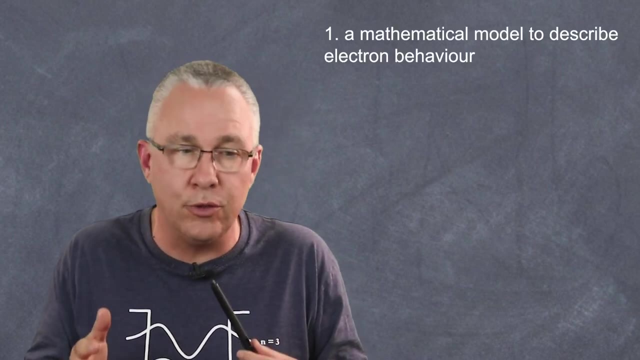 And this is the key point I want to leave you with after taking you through all that. Number one: we have a mathematical model to describe how the electron behaves around the educate. Secondly, this particular model can also apply to other atoms. Now, I've just